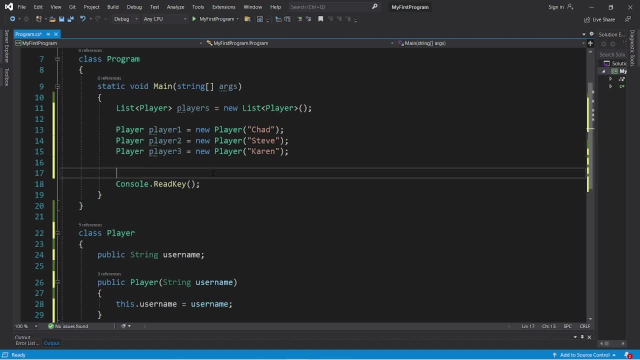 what about Steve and Karen? Okay, now to add our player objects to our list. type the name of the list: dot add, and then pass in the name of the object Players- dot add Player1,. then do the same thing with player2 and player3.. Then I'll use a foreach loop to display. 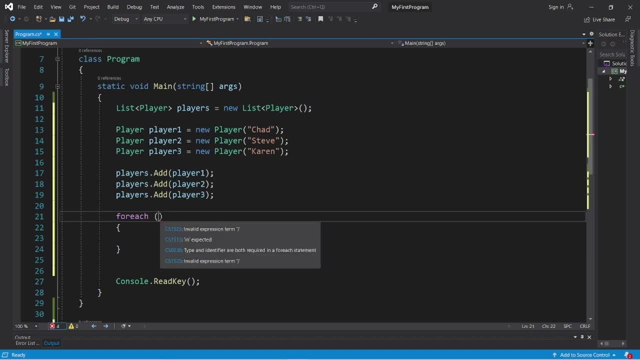 all these Foreach, the data type is player, player in players. So let's take a look at this. I'm going to consolewriteline each player, But since we're displaying each object directly, what's going to be displayed is the namespace plus the data type. 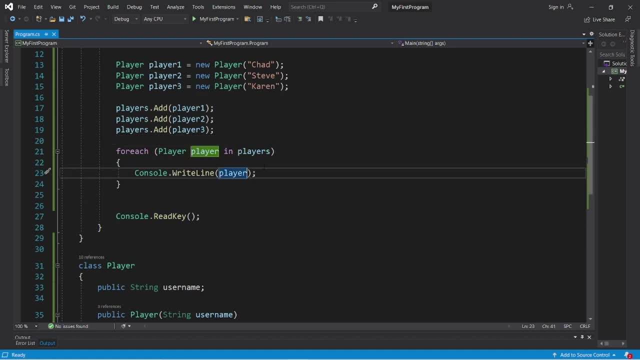 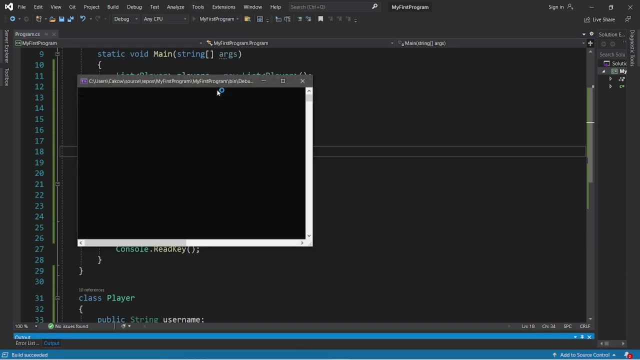 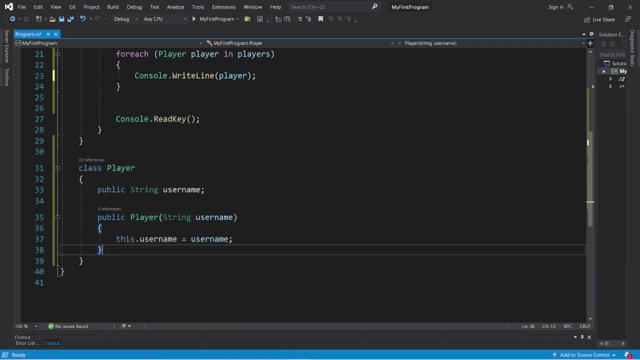 our object. We can access the username field And that will display each player's username, Or we can override the toString method, So we have Chad, Steve and Karen, Or we can override the toString method, So let's try that too: Public override toString And I'm going to return username. 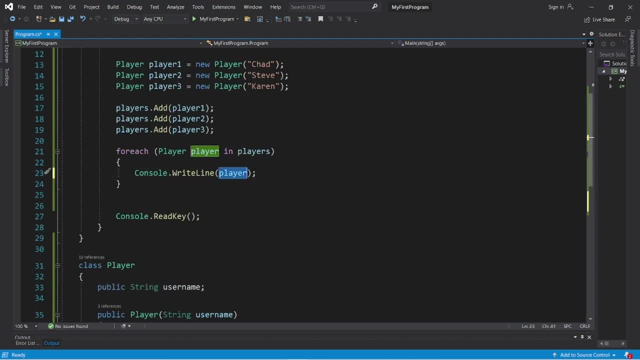 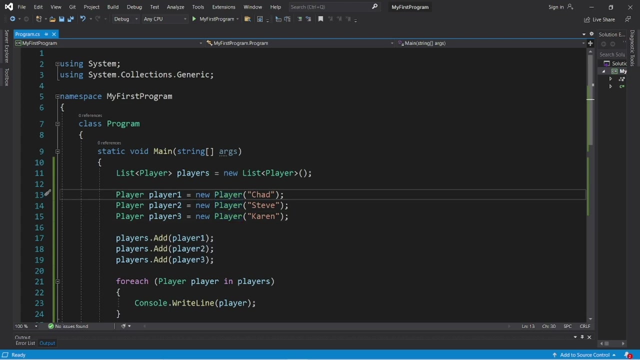 So then when I use consolewriteline, I can just type in the object's name. So we have Chad, Steve and Karen. Now another thing that you can do: when we instantiate these player objects, we can do so anonymously. So within the add method of our list players. 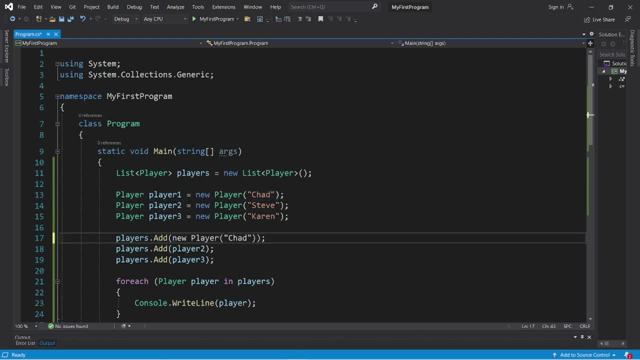 we can simply just pass in new player, then pass in a name, And then we don't necessarily need to create a name for each of these objects. So I'm going to pass in new player Steve and new player Karen. So this is optional, but I like to create anonymous objects. 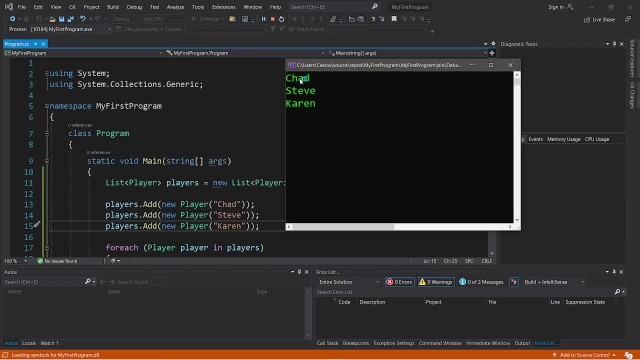 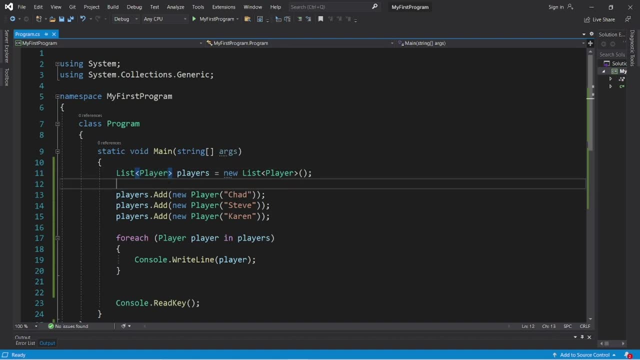 It's less work. So we should have our three players, Chad, Steve and Karen. So yeah, that's how to add objects to a list. Within the angle brackets, you just list the type of object that you would like to store within your list. So yeah, that's a list of objects in C sharp, If you. 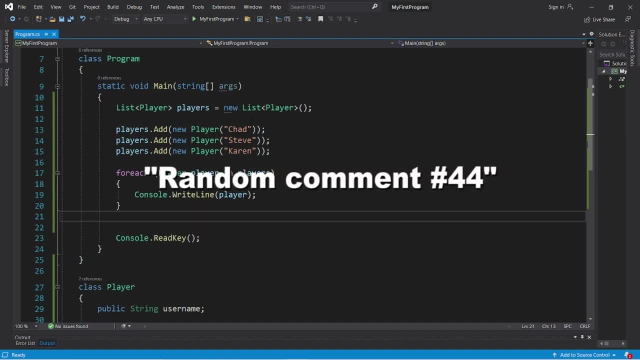 found this video helpful. please be sure to smash that like button, leave a random comment down below and subscribe if you'd like to become a fellow bro.